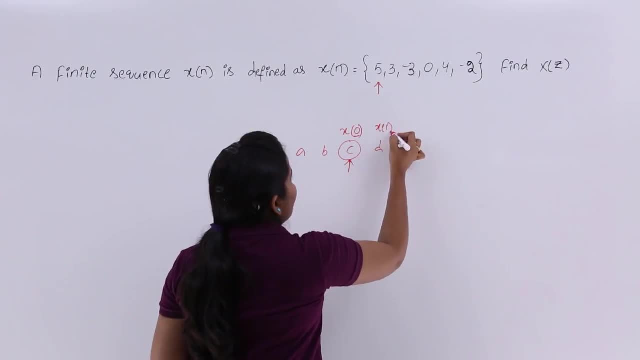 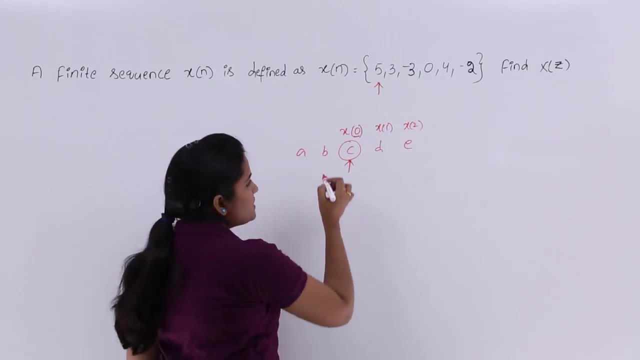 as right sided sequence, like x of n and x of 2. like this, The sequence is completely right sided because our sequence is fixed like this. So in that example there is a elements left to this x of 0. you need to consider like x of minus 1 and x of minus 2, up to x of. 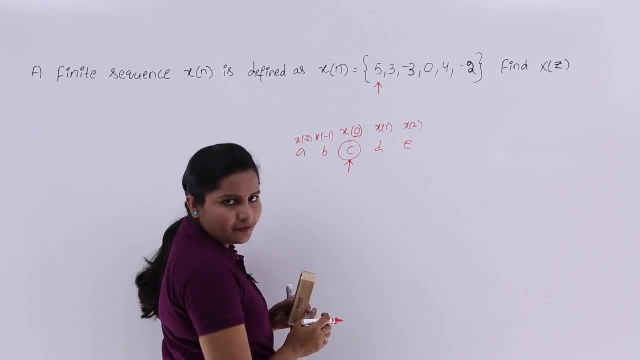 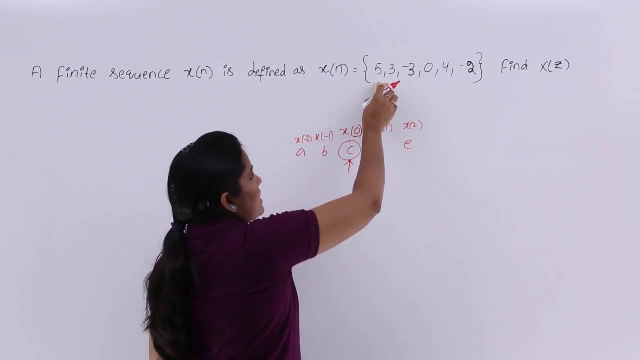 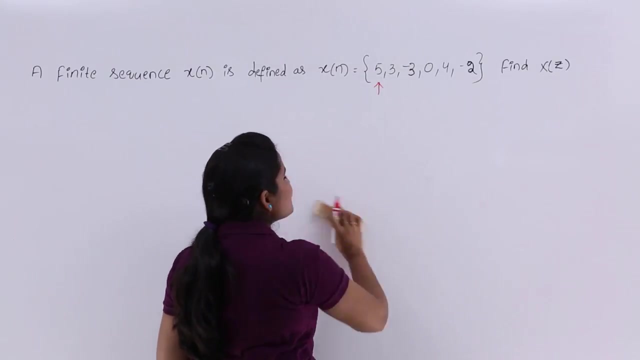 minus infinity this side up to x of plus infinity, like this way we need to consider: if arrow mark is not given, you need to consider: starting point is the x of 0. that means you need to consider your sequence as fully right sided sequence. so here you are, having this as x of 0 and this as. 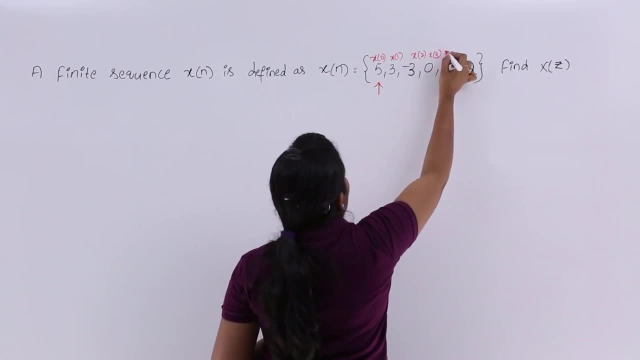 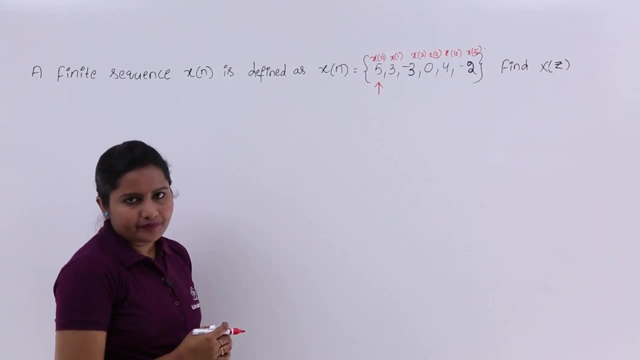 x of 1, x of 2, x of 3, x of 4, x of 5. so you need to consider: up to n is equivalent to 5. starting from n is equivalent to 0 to 5. you are having your signal, what they are asking. 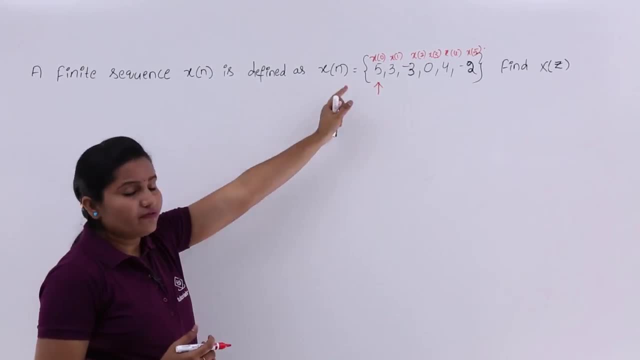 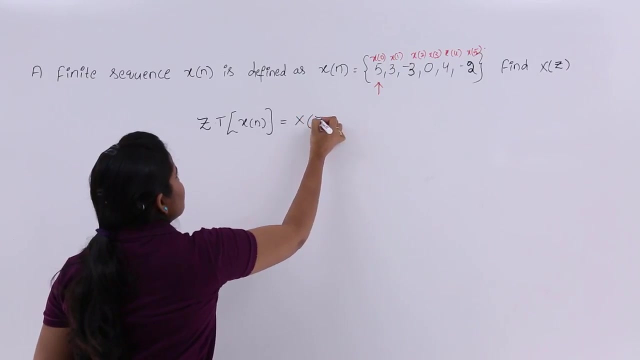 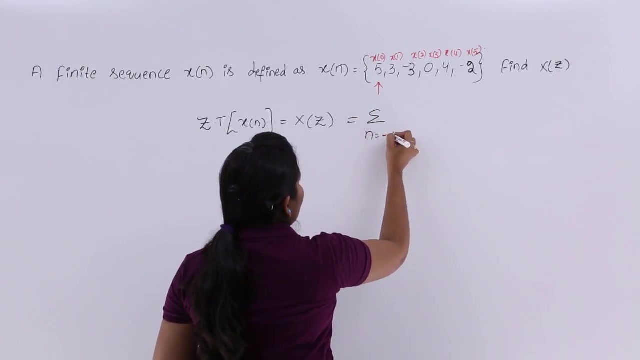 they are asking: what is the z transform of the finite duration sequence? x of n. so now i am writing that z transform equation. they are asking: what is the z transform of x of n? so z transform of x of n is always represented with x of z. so this x of z is equivalent to summation, n is equivalent to minus infinity. 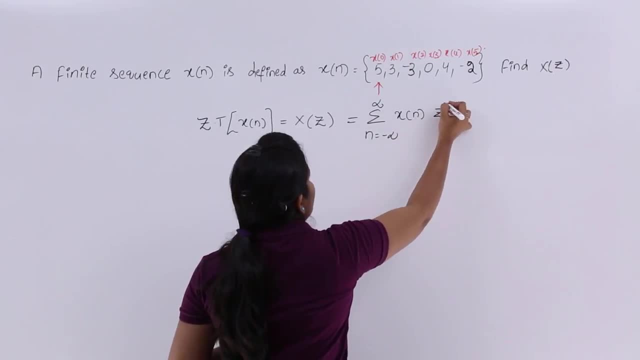 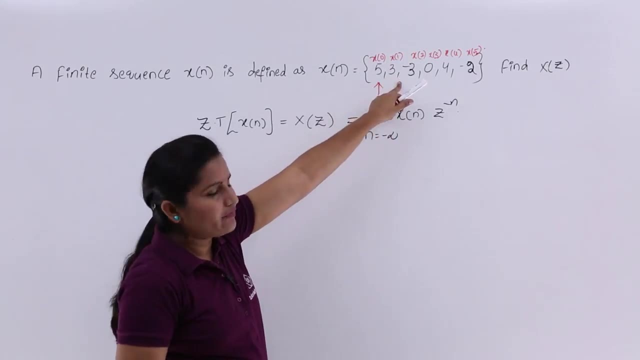 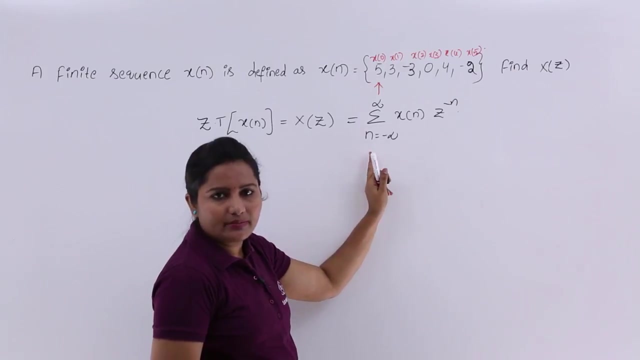 to infinity, x of n into z power minus n. this is the equation for z transform of any signal x of n. Here we are having our signal x of n. we are having our finite duration sequence here, so by that we can limit this limits. n is equivalent to minus infinity to infinity. here we are having 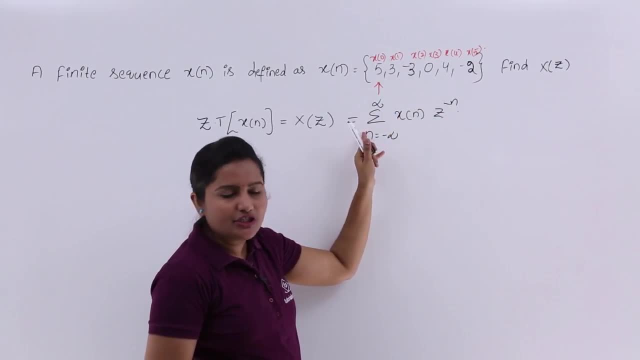 so by observing the sequence itself, we can limit this summation to: n is equivalent to 0 to 5. why? because if you consider minus infinity to infinity also, you are not having your signal. x of n. that means minus infinity to 4. your x of n is equal to 0. 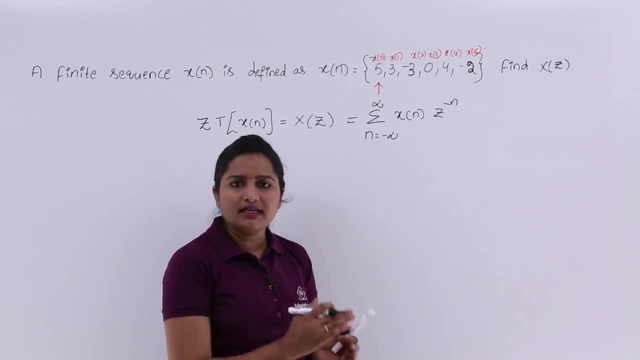 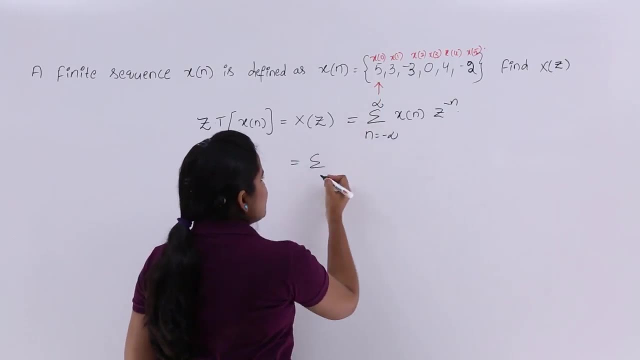 you are not having any sample means your value for that signal in that region is equivalent to 0.. So now that is why no need to take any other regions, only required region. you need to consider 0 to 5. they given up to 0 to 5 x of n z power minus n. 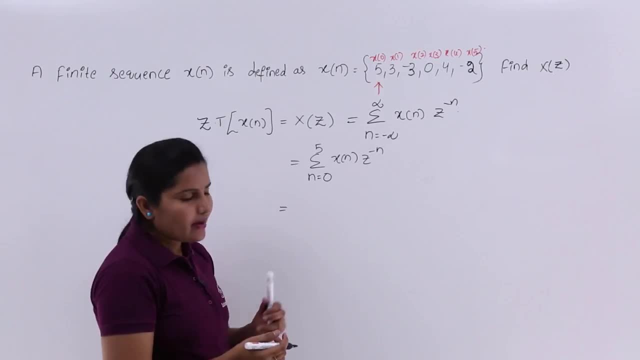 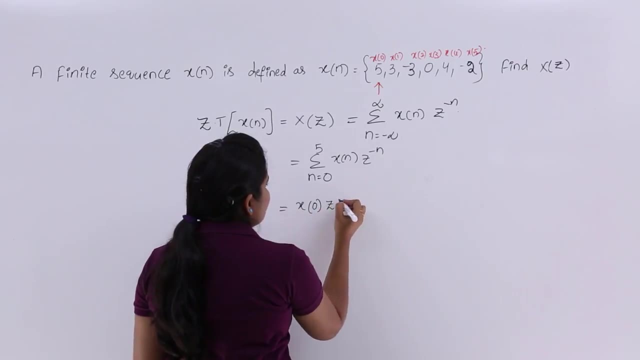 Now i am expanding this sequence, so this equation says 1 x of n minus infinity to 4 x of n is. I am expanding this summation, just. I am substituting n equal to 0 here x of 0, z power 0 in place. 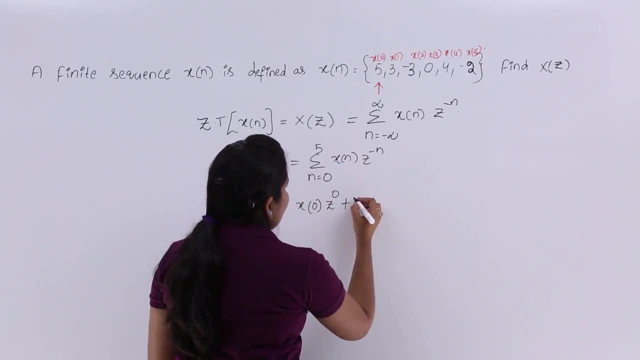 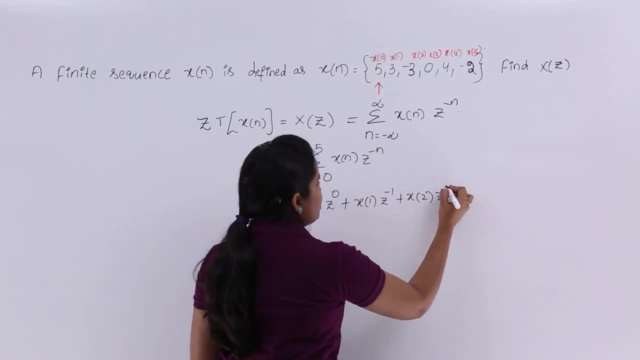 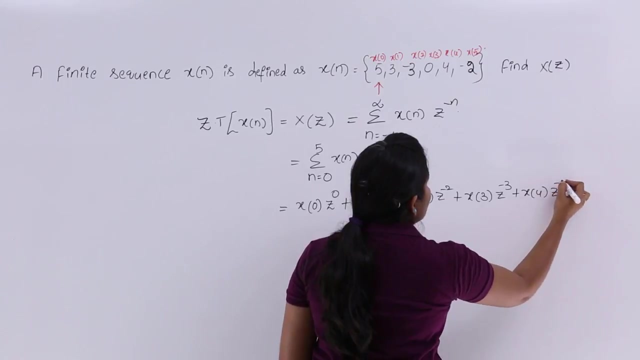 of n. I am substituting 0 plus here. n is equivalent to 1 x of 1 z power minus 1 plus x of 2 z power minus 2 plus x of 3 z power minus 3 plus x of 4 z power minus 4 plus x of 5 z. 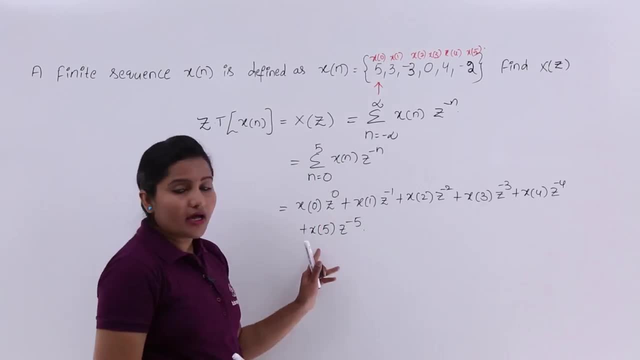 power minus 5. so up to n is equivalent to 5. I expanded this summation. in this sum, in this values we know x of 0, x of 1, x of 2 and x of 3. if I substituted that values, you are going to get your z transform of the sequence x of n. 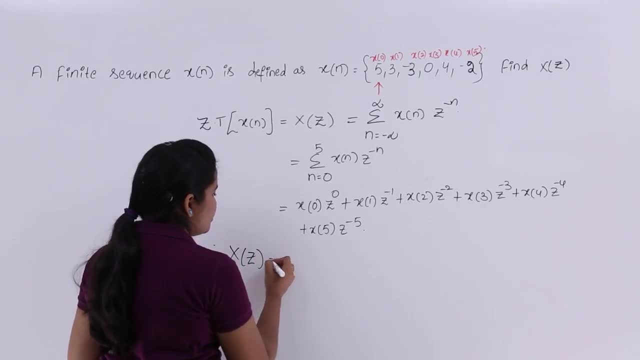 So therefore x of z is equivalent to: for the given sequence, x of 0 is 5,. 5 into z power 0, no need to mention z power 0 is also equivalent to 1, so plus x of 1 means that is equivalent. 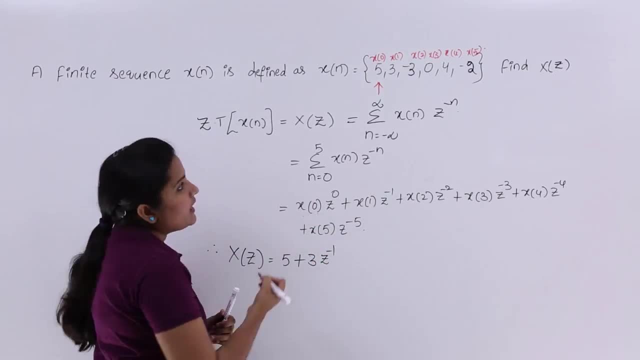 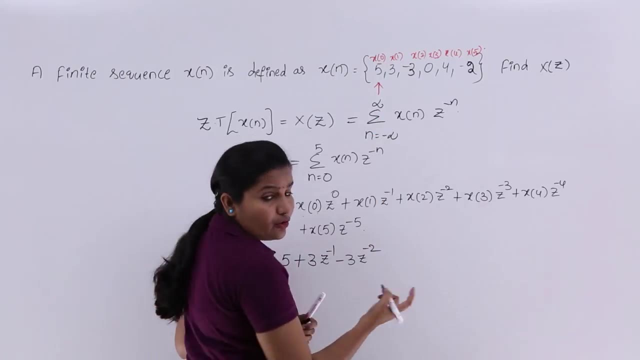 to 3 into z power minus 1 plus x of 2, value is a minus value minus 3 into z power minus 2 plus x of 3 is 0,. 0 into z power minus 3, you will get 0.. 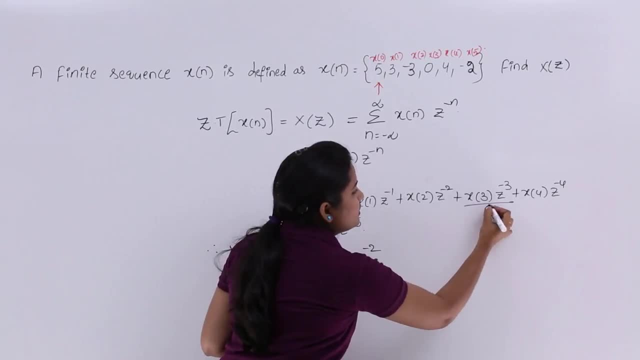 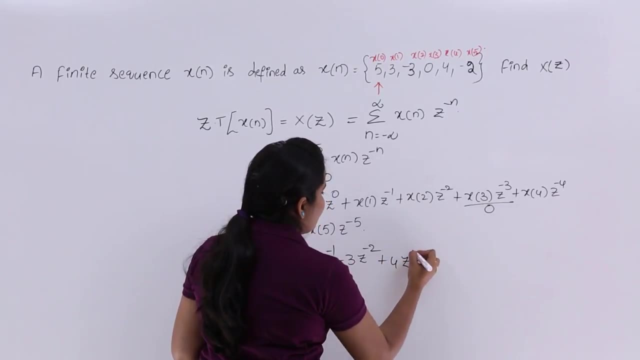 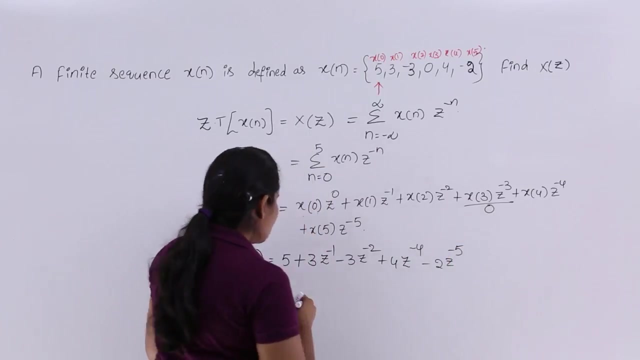 So I am not going to consider this value. why? because this value is going to be 0 plus x of 4. value is 4, 4 into z power minus 4. finally, we are having x of 5, again negative value- 2 into z power minus 5.. So this is the z transform of given sequence like this: 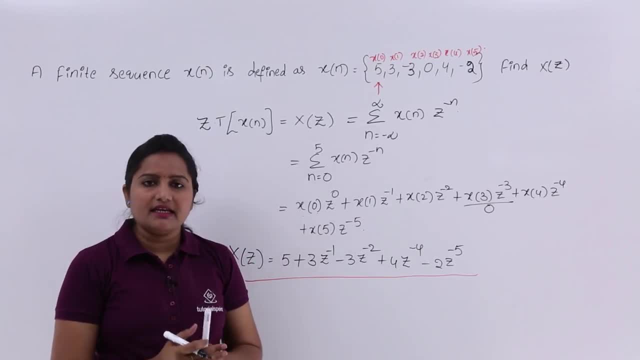 way we need to get the z transform of discrete finite duration sequences.